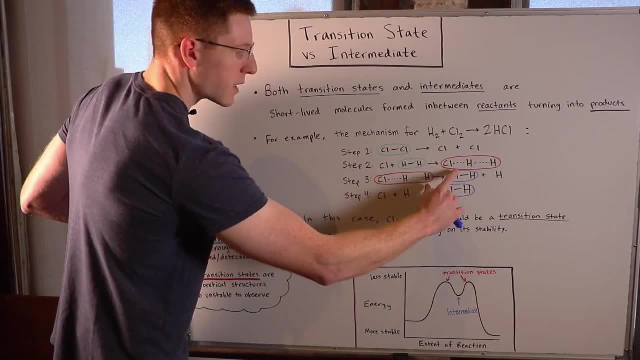 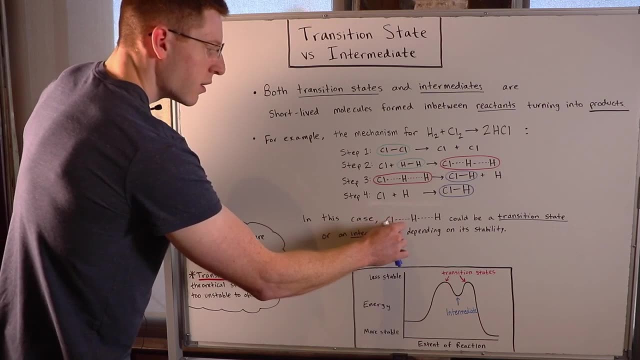 at this more closely. Subtitles by the Amaraorg community. But you can see that we form something in the middle in red here that is then destroyed before we get to our products, In this case this ClHH here with this sort of half bond. 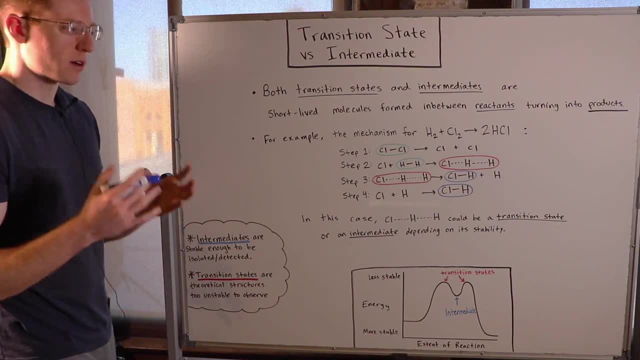 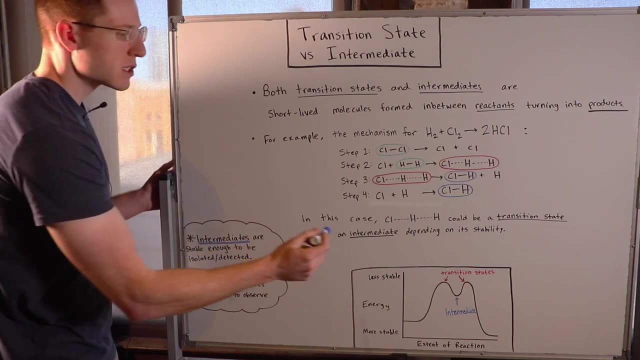 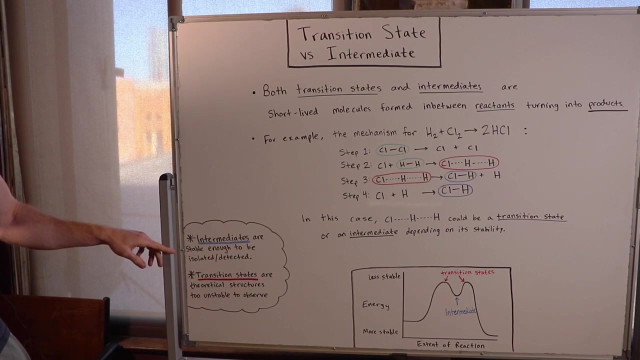 that's not completely a bond, but you can see the atoms are still interacting. in some sense. could be a transition state or an intermediate state, And we determine that based on its stability. So intermediates are actually stable enough to be isolated or detected. 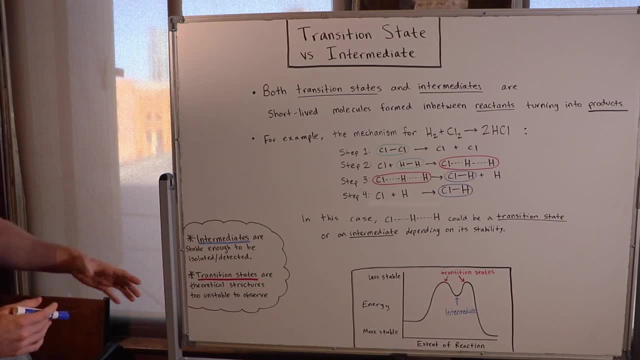 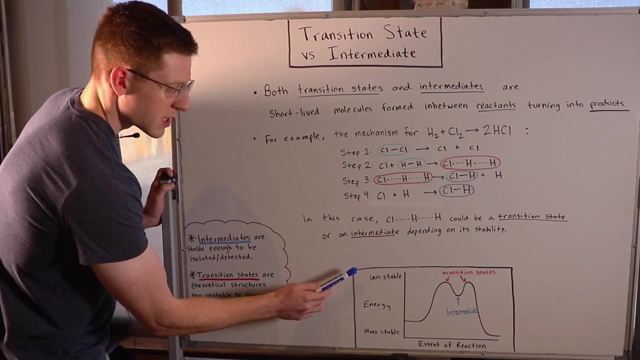 while transition states are theoretical structures that are too unstable to actually observe. We sort of hypothesize what they should be as a transition state, but we can't actually look at them in the laboratory. So I've presented these graphically down here. You can see on the Y axis I have energy, So 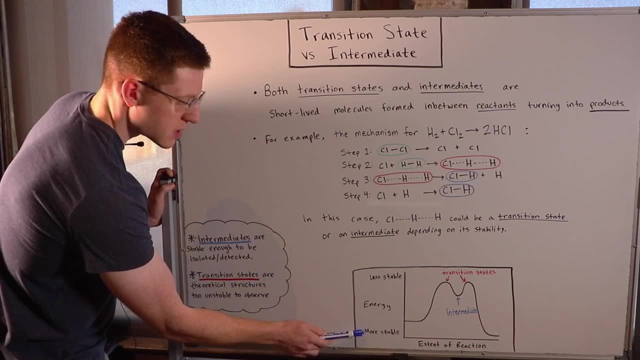 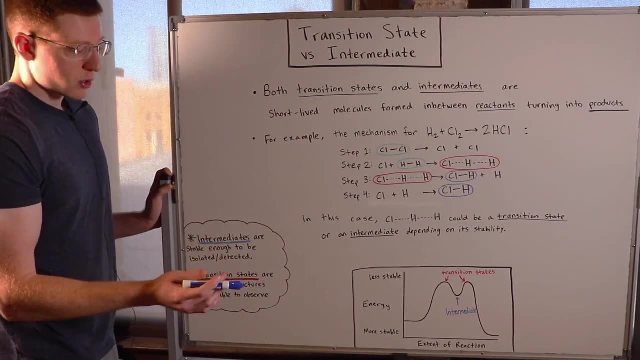 up here is highest energy or the least stable state, and at the bottom is lowest energy or the most stable state On the X-axis. I have the extent of my reaction and this is what a general reaction coordinate looks like. Put a bit of более general, but this is much more basic structure, So you may want to look at it from this point. 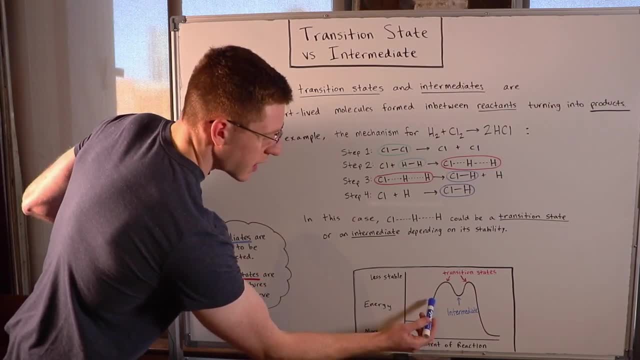 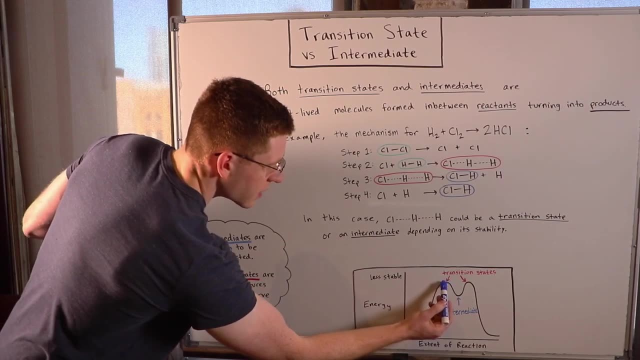 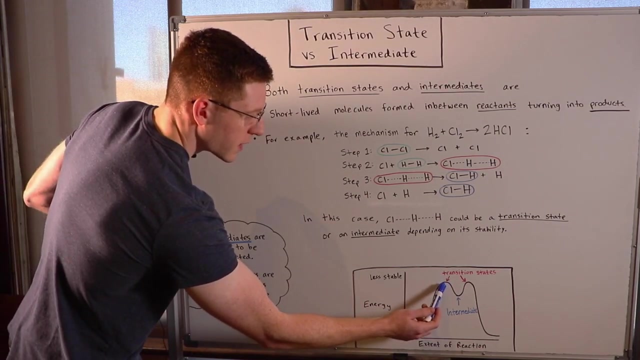 We start out with our reactants. we increase in energy and a hump here or the top of the hill represents a transition state. This is the highest energy point and remember transition states are very unstable right, The higher the energy, the more unstable you are. 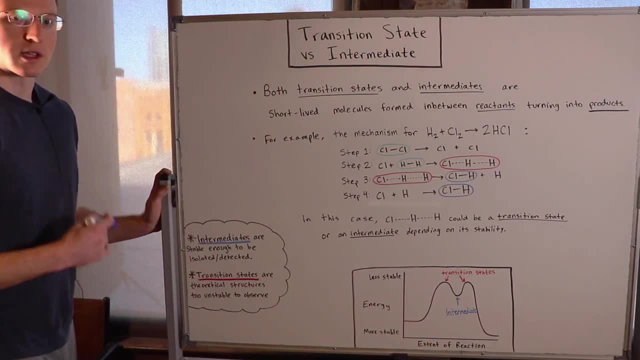 Then we go down into a valley here or a dip, and this represents an intermediate. You can see it's got lower energy and it's more stable than the transition states and it's actually stable enough to be isolated or detected or somehow observed. 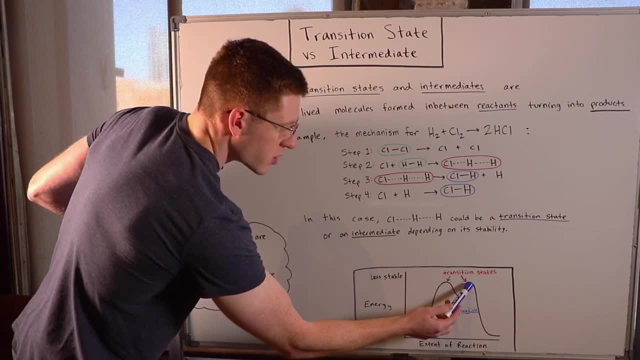 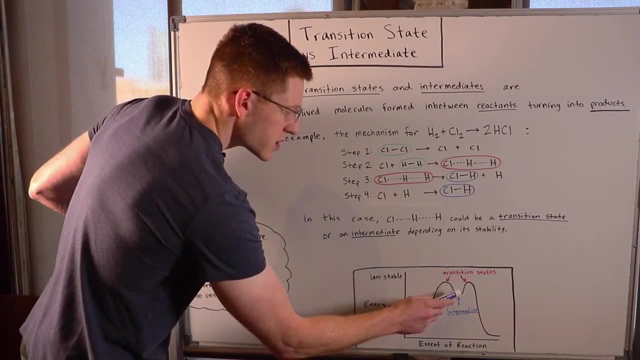 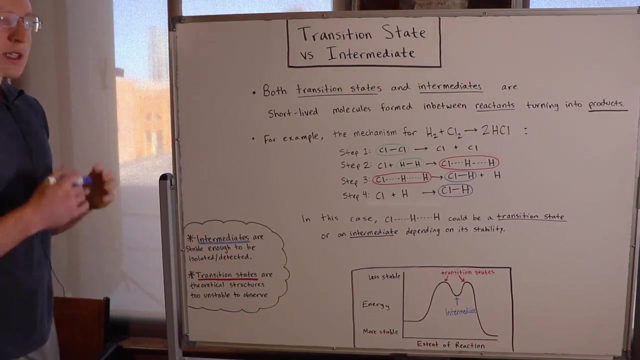 Then we increased again and got up to another hill or a hump, to a transition state, and finally we fell back down and reached our products. So you can see here that transition states and intermediates happen in between turning reactants into products, and the difference between them is their stability. 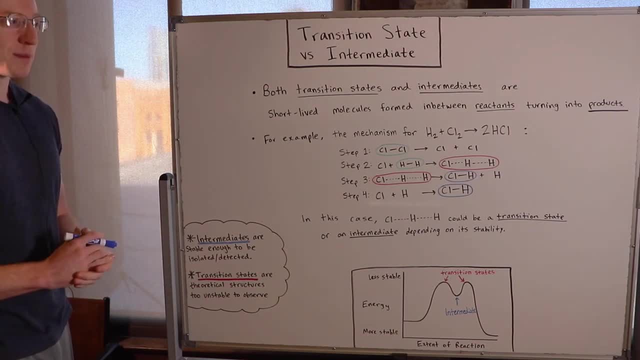 So I really hope this video helped you guys out. if it did, please feel free to give it a thumbs up, and I'll see you in the next one.